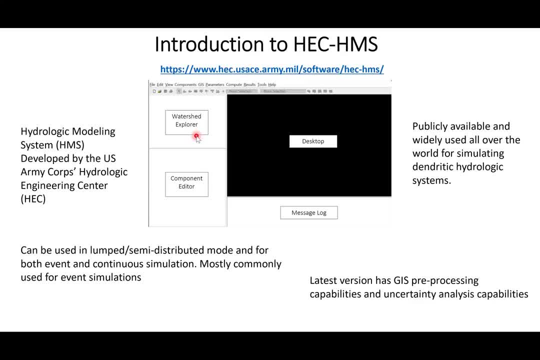 Watershed Explorer will show you what is included in the model. So if you have Base, it will show the name of that basin. If you click on that basin it will show you what is included in that basin model. If you have Time Series, you will see that time series file or folder here. and 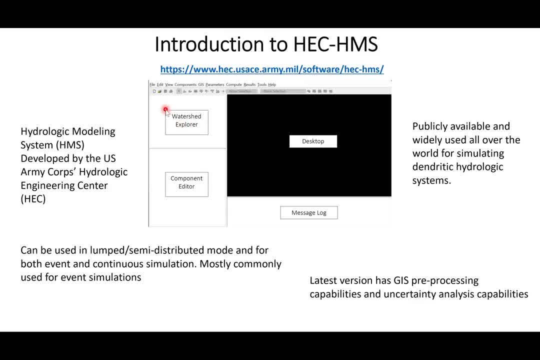 when you run simulation- this is where you can find what the simulation name is, and so on- And when you select something in the Watershed Explorer, the parameter associated with any element or information associated with any file is shown in the Component Editor. and when you run simulation, 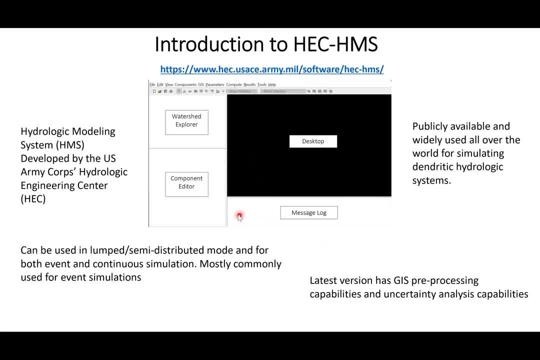 when you do something in your HEC-HMS model, all that information is displayed here in the Message Lock. So if you run a simulation and get an error, this is where you will see. So again, this is just a quick overview of HEC-HMS interface, So let's move on to learn more about HEC-HMS In order to 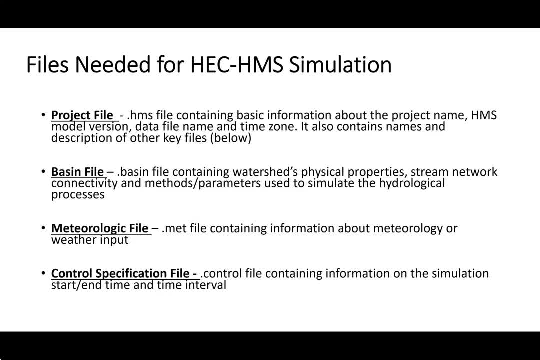 perform a HEC-HMS simulation, we need to have these four files. So when we say we create a HEC-HMS model, basically we are creating these four files. So the first file is project file and it will have an extension of hms. So whenever we create an empty HEC-HMS model and save it, a hms file will. 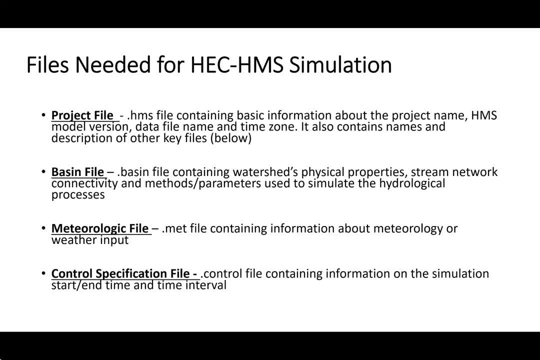 be created and it will contain information about the project. It will have a project name and it will have that project name. It will also have the model version and it will also have the data file name and time zone, and it will also contain information about all the related files, which are: 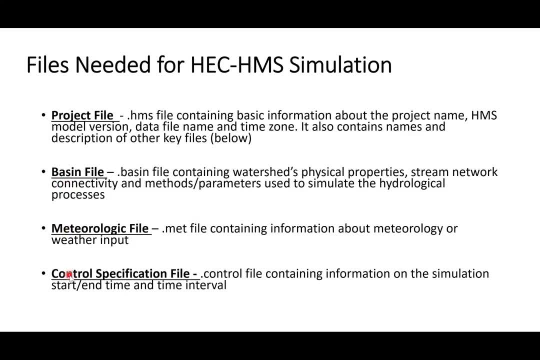 these three files: Basin file, meteorologic file and control specification file. Basin file will have an extension of basin and it will basically contains watersheds, physical properties, stream network connectivity and methods and parameters used to simulate the hydrological processes in the model. Meteorologic file will have a met extension and it will contain 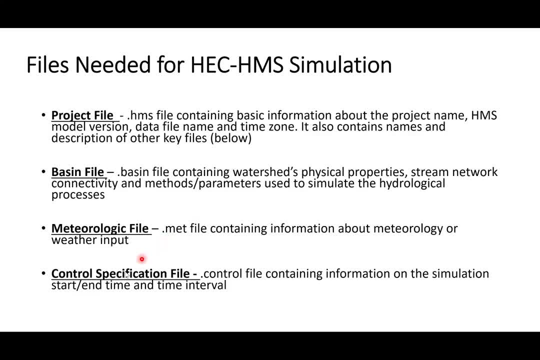 information about meteorology or weather input. And finally, control specification file will have an extension of control and it will contain information on the simulation start date, end date and time interval. So let's quickly look at the details of some of these files and we'll spend more time talking about the Basin file. 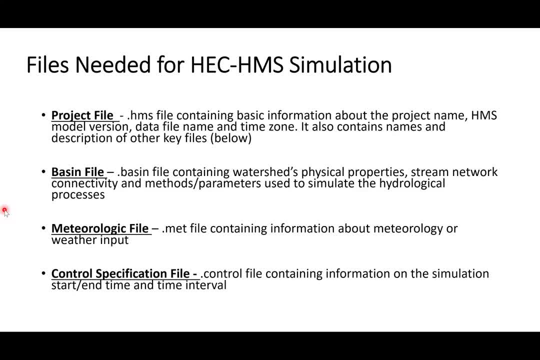 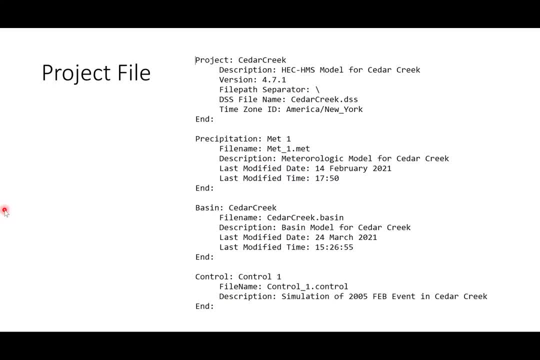 because that is the important file that you need to run a HEC-HMS simulation. This is how a project file looks, So you can see it is a text file, so even though it has an extension of hms, you can open that using notepad. It has this basic description, including the name, version data file. 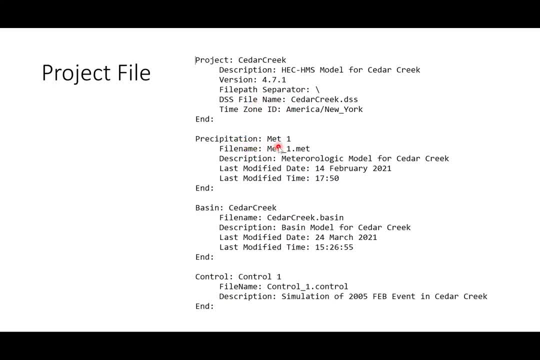 time zone. and then there is this meteorologic file that has a name of met, underscore one. You have the basin file. This is for cedar creek, so this is cedar creek dot basin. and then this is the control specification file, which is control underscore one, So project file. 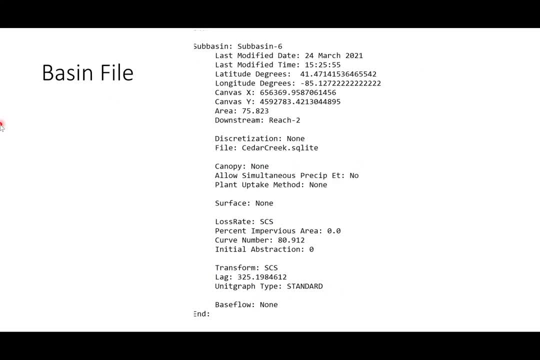 is simply a text file. Next we have basin file. So what you see on this slide is just a small portion of what the basin file includes. So what you see here is information about a sub-basin. It has a name, sub-basin dash six. This includes the information on its location, its area and 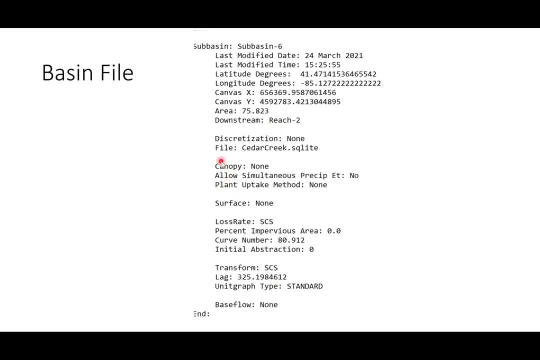 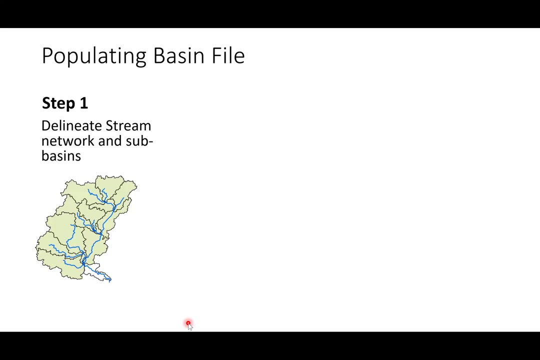 what is downstream of that basin, Then it will contain information about the methods that are used to simulate the hydrologic processes in that basin, and then this information will be repeated for all the sub-basins, and then it will have similar information for all the reaches and junctions and so on. When we create basin file, it will be an. 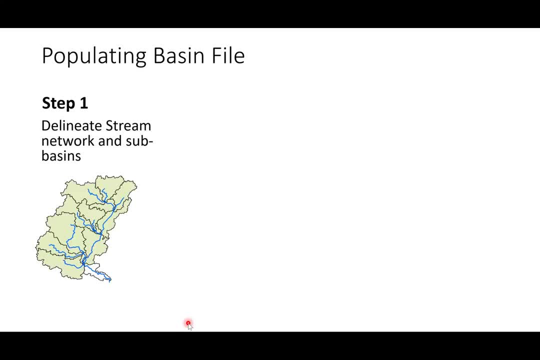 empty file. so we have to populate that basin file. and there are three steps involved in populating that basin file. The first step is to delineate stream network and sub-basin. So remember, basin file contains properties of our watershed and to extract those properties we have to delineate stream network. 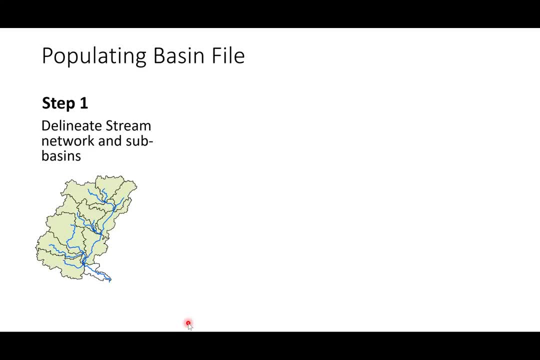 and these sub-basins. We know how to do this, using ArcGIS, hydrology tools and also ArcHydro, and in older versions of HEC-HMS we did not have any GIS capabilities, so we had to use, for example, GeoHMS to do all this, but these days, with newer version of HEC-HMS, we don't. 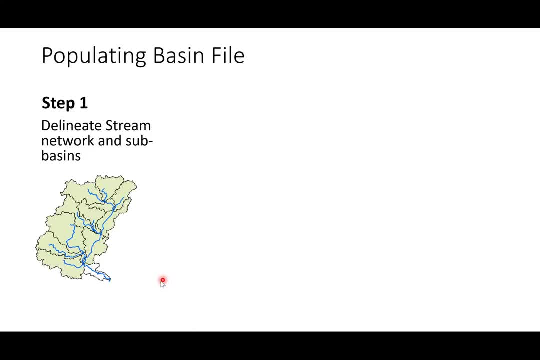 need any other external GIS program to do that. So we are going to use the internal GIS capabilities in HEC-HMS to perform this first step. After that first step, we move on to step two. So in step two, we will select each of these sub-basins that you see here. when, for all these reaches, we will select. 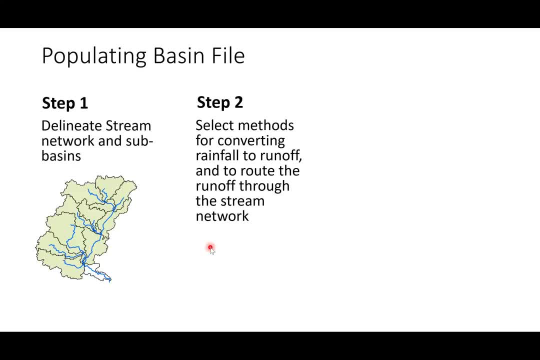 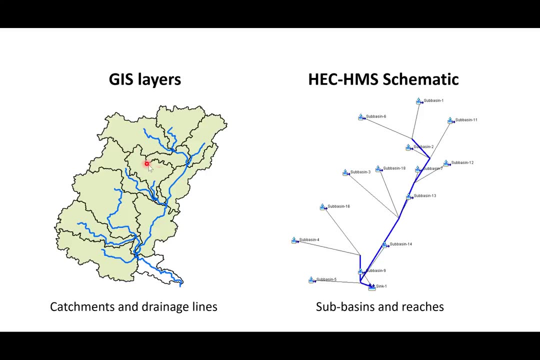 some methods to simulate the hydrology, and then, finally, in step three, we will assign parameters to all the methods that we have selected in step two. Now, HEC-HMS is a computer software, so even though our sub-basins and river network look like this, but the program doesn't have the 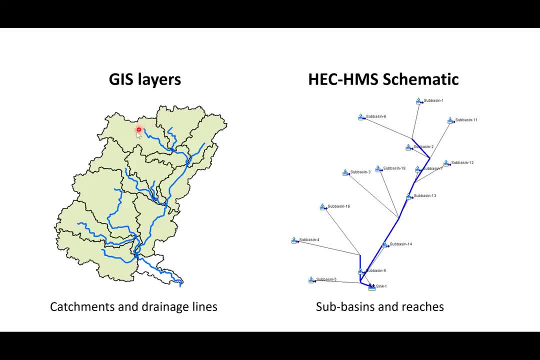 exact shape of all these sub-basins and streams. All it cares is about connectivity. So instead of using these GIS layers, HEC-HMS will create its schematic network, and this is what you see here on the right. So what we have are the sub-basins that are representing these polygons, and then this: 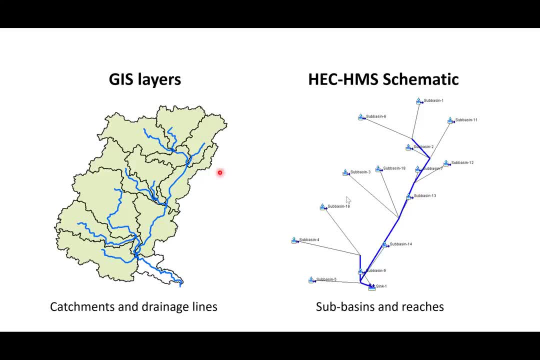 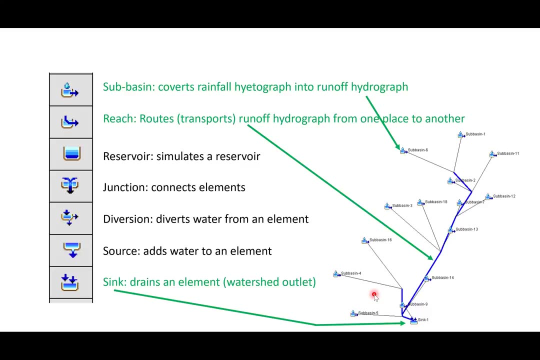 dark blue line that you see here are the sub-basins. So these are the streams that are connecting all these sub-basins and finally, we have this sink, which is our outlet. So there are multiple elements in HEC-HMS that we can use to represent the 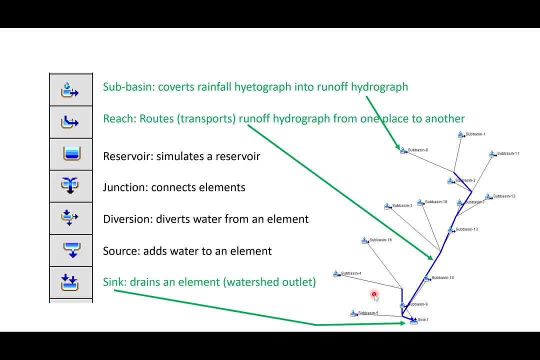 hydrologic system In this module. we are not going to use all of them. We are mainly going to use sub-basins that we saw in the previous slide, and these sub-basins are connected by reaches, So we finally everything drains to the outlet, and that outlet is represented by a sink in HEC-HMS. 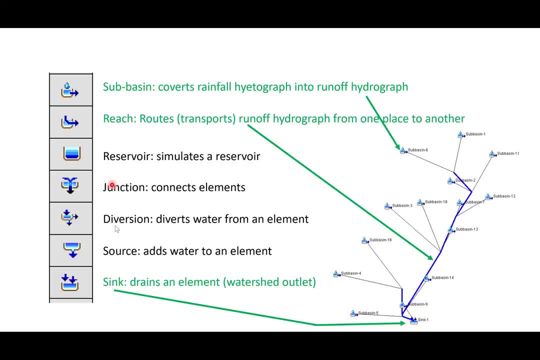 So if we include reservoirs and diversions and if there is a source that is adding water to our watershed, we can add these other elements. but in this module we are just going to create a simple HEC-HMS model, So we will only use sub-basin, reach and sink. So sub-basin is a 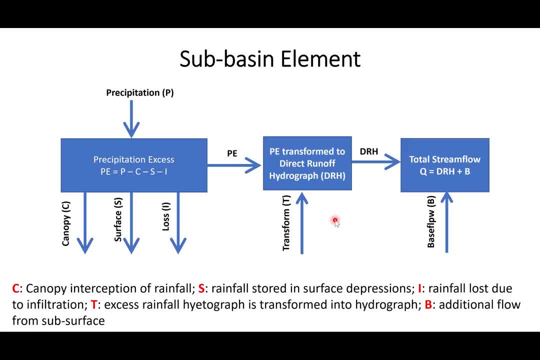 very important element in HEC-HMS. This is where the rainfall gets transformed into runoff. So the key input here is precipitation, and after that precipitation falls on a sub-basin, the program will calculate excess rainfall. So in order to calculate excess rainfall, the program should know: 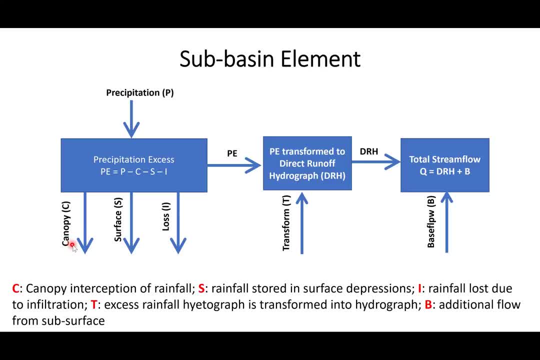 where all the water is getting lost. So there are methods to incorporate those. So the first one is surface processes, So this includes the water that gets intercepted by trees and other vegetation on the land. Then we have surface processes or methods, So this represents any sort of depressions. 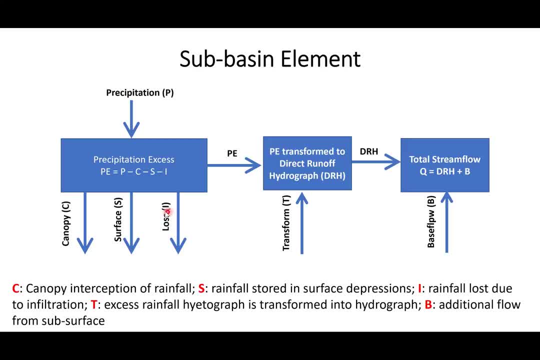 and storage that we have on the surface. And finally, we have loss methods. So loss in this case represents the water infiltrating into the ground. So these are the methods that we can use sub-basin to convert precipitation into excess rainfall or excess precipitation. 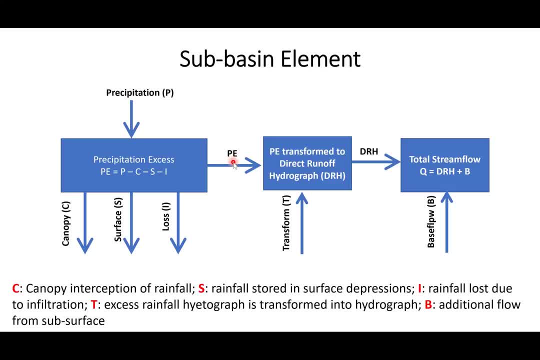 or direct runoff And from that direct runoff we will create the hydrograph and that is performed using a transform method. So excess rainfall is transformed into direct runoff and once we have that direct runoff we can add base flow to get the total stream flow. So these are the processes that are involved at the sub-basin level. 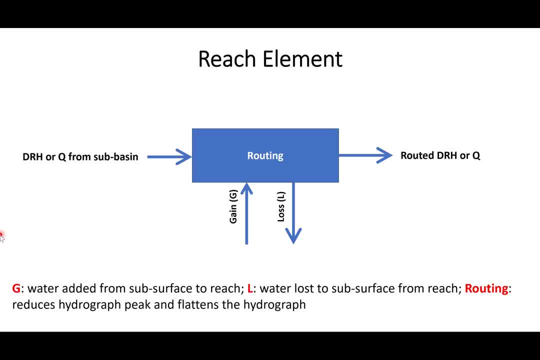 After we get the hydrograph from the sub-basin, it will flow through those reaches to reach the outlet. So essentially, when the water is flowing through those reaches, we perform routing and then we also have loss and gain methods. So if the water is getting lost as it is flowing through, 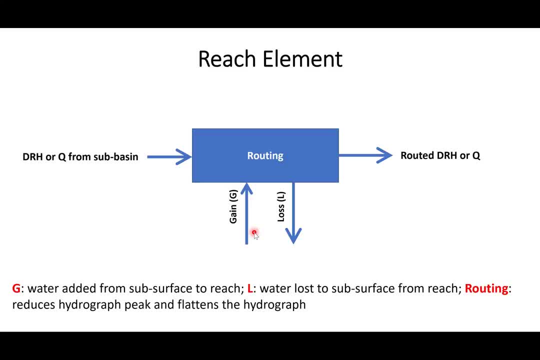 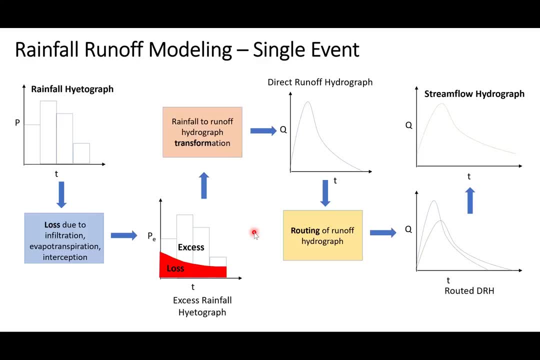 the source or if it is gaining water, then we can incorporate that. This is a graphical view of all the processes that are taking place as the rainfall gets transformed into stream flow. So we start with rainfall hydrograph, which is the main input, Then we calculate loss and then after. 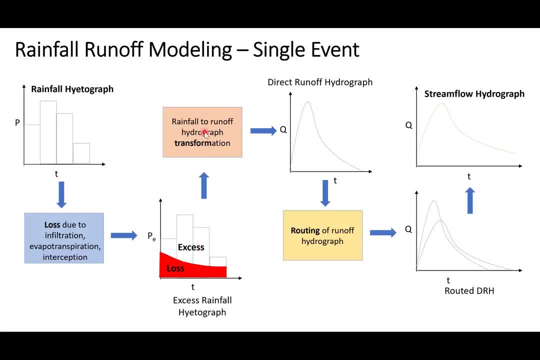 subtracting that loss, we get excess rainfall transformed into direct runoff hydrograph, and then that direct runoff hydrograph is routed through reaches to get the routed hydrograph and finally we can add base flow to get the total streamflow hydrograph. now, these are all. 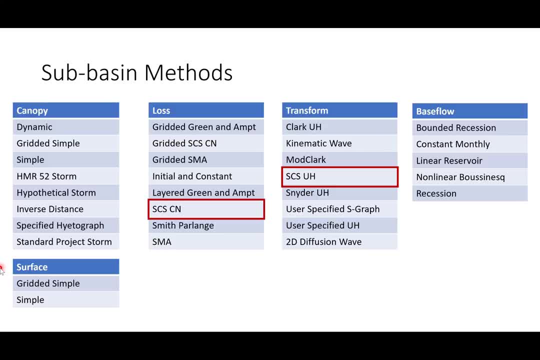 the methods that are available in HEC-HMS and we are not going to use all of them. we are not going to use canopy, we are not going to use surface, we are going to use loss and to perform that loss we are going to use the SCS curve number method. 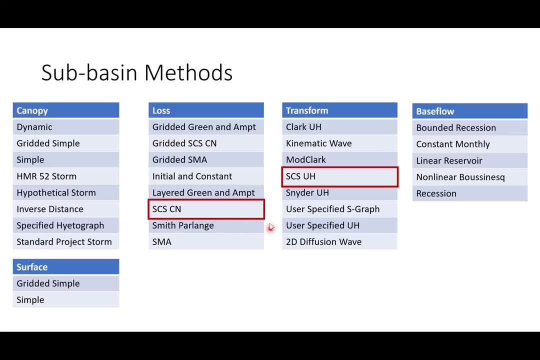 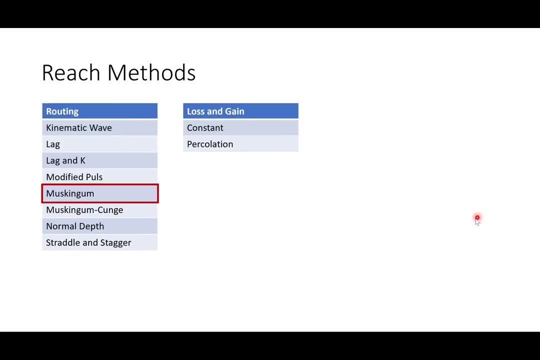 to get excess rainfall. and then we will transform our excess rainfall to direct runoff hydrograph using the SCS unit hydrograph transform method and again, we are not going to include any base flow for reach. these are the routing methods that are available to us in our case. 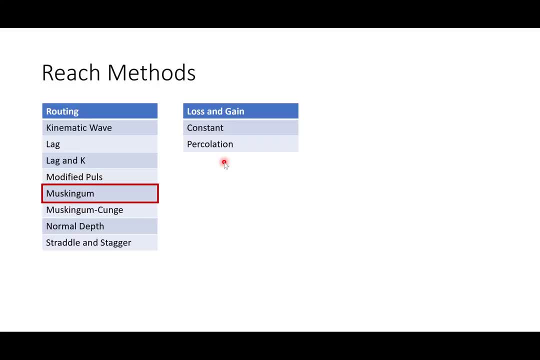 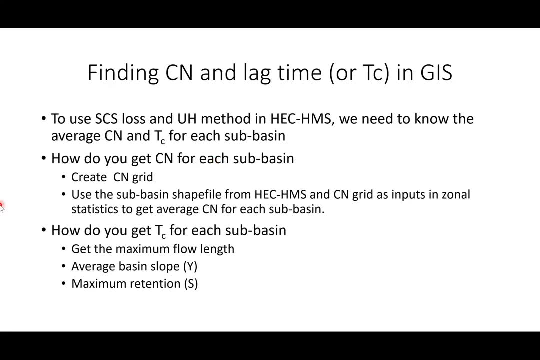 we will only use Muskingum method and we are going to ignore loss and gain methods. now, as I mentioned earlier, we had to use a GIS interface to create a basin file, but the late version of HEC-HMS has GIS capabilities. it is still evolving so it does not have all. 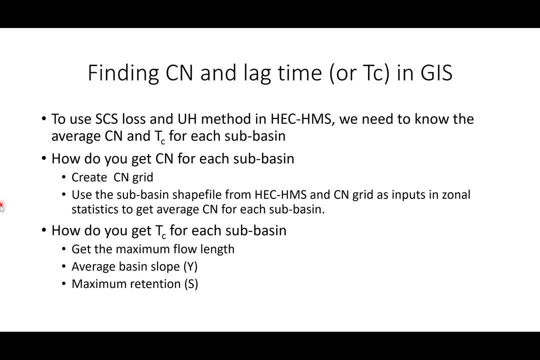 good hoping for the duration of the data, and i will leave this here. for the capabilities specifically does not have capabilities to extract some of the parameters. so the two parameters that are critical for the SCS curve number method are the curve number and then for the transform method we need to get the 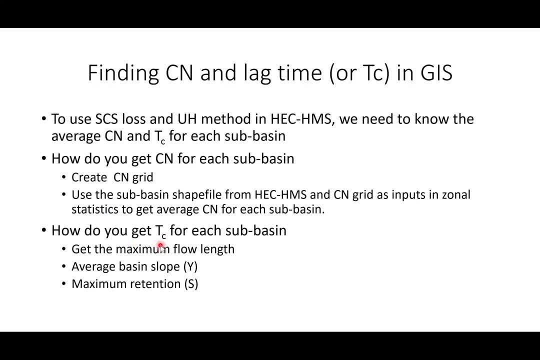 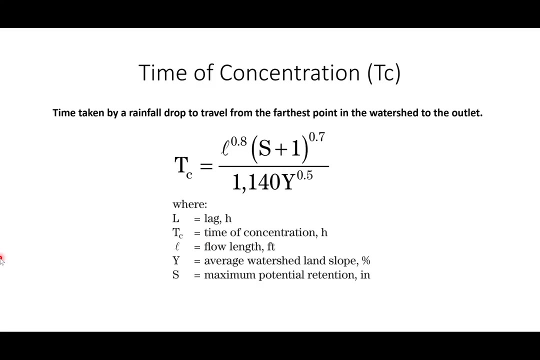 lag time, or that lag time is dependent on time of concentration. so here is a brief methodology on how to do this, and when we actually create the model, we will see how to perform these steps in detail using example data sets. this is the equation that we are going to use for calculating the time of 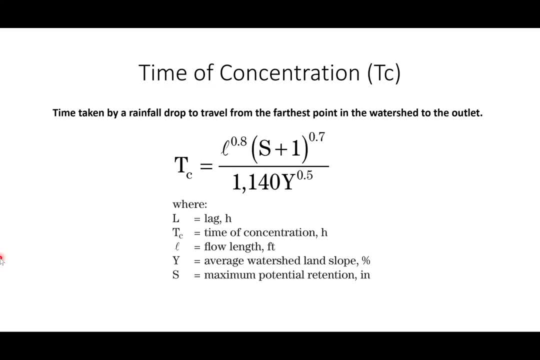 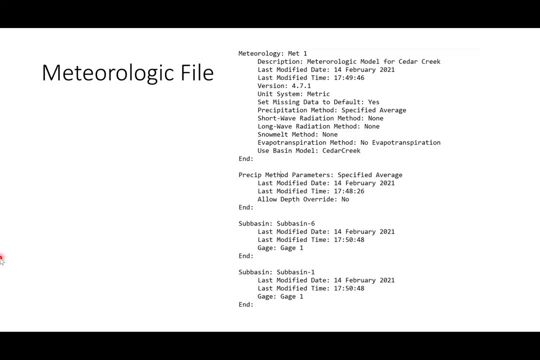 concentration, which will then be used to calculate the lag time, and we are going to see how to use this equation in HEC-HMS by also using HEC-HMS, using some GIS capabilities outside HEC-HMS. after we have basing file, the next file that we have to create is meteorologic file, as I mentioned. 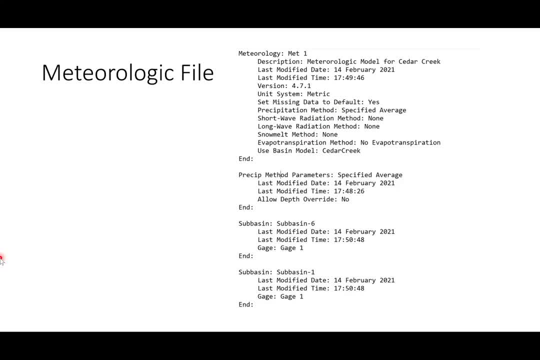 meteorologic file will include information on weather input, and this is how a meteorologic file looks like now. this file does not necessarily contain all the rainfall values, as you can see here that the rainfall information is stored in another file called gage1, so this is a time series file and we are going to see 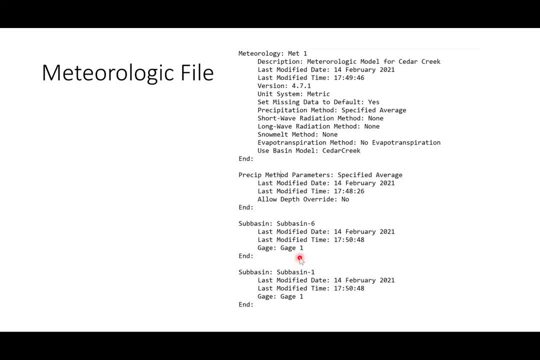 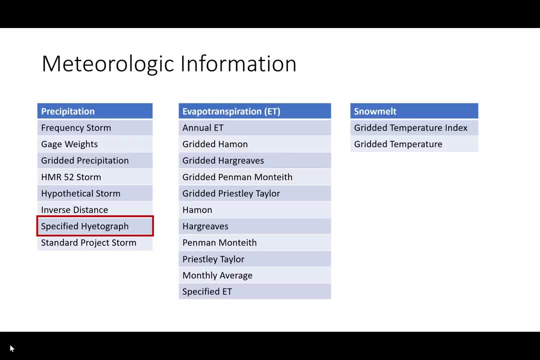 how to create that time series file when we create our HEC-HMS model, similar to the sub basin methods. there are multiple options for including meteorologic information and you see three options here. one is for precipitation, the second one is for evapotranspiration and the third one is for serve basin Showers. we are going to show as three. 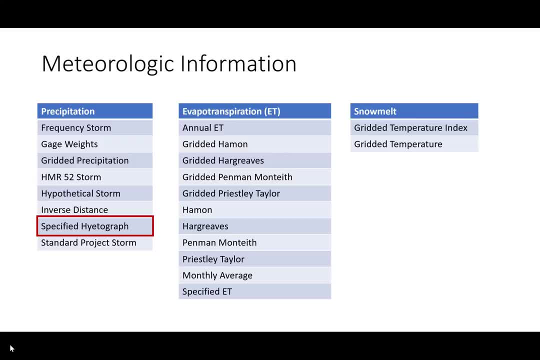 of theseveer. the third one is for evapotranspiration and the fourth model is one is for snowmelt. in this model, we are going to perform hydrologic simulation for a single event, so we do not have to worry about evapotranspiration and 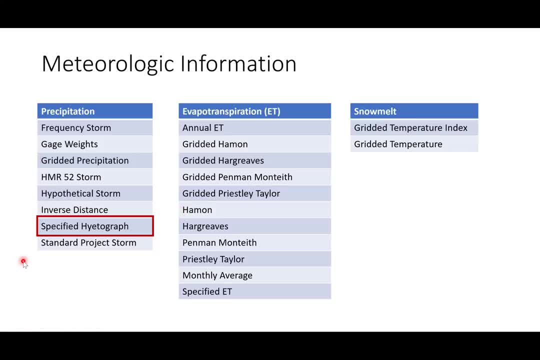 snowmelt. so we will only use precipitation information. and again, for specifying precipitation, there are multiple ways. in our case we are going to use specified high-altograph and we will specify that high-altograph by creating a gauge. after you create meteorologic file, the last file that we